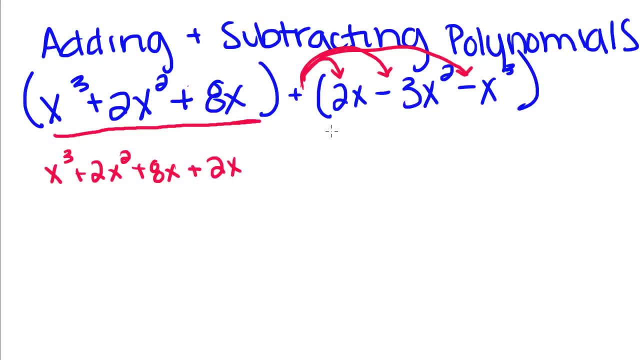 stays the same, and this is plus 2x. and positive times negative stays negative, 3x squared. this also stays negative, 3x cubed. And now what we're going to do is you can do two different things and it just depends on what you prefer. better You can write it in descending order. 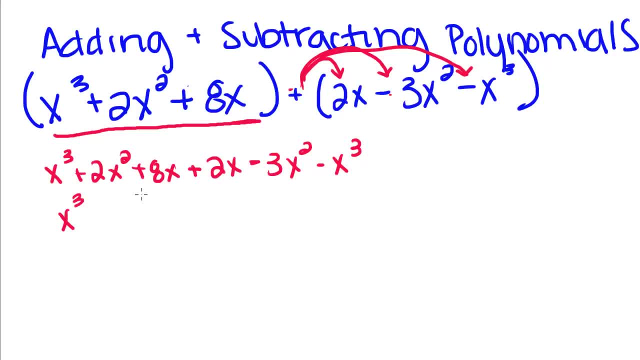 so you have your highest power and then we're going to bring this one over and then your next highest power. If you want to rewrite it before you combine your like terms, you don't have to. I personally don't, but it really doesn't matter what you do. So x cubed minus. 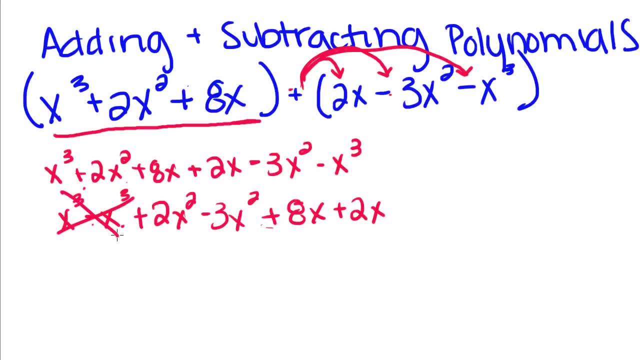 x cubed is 0, so those are going to go away. 2x squared minus 3x squared is going to give us a negative x squared, and 8x plus 2x is going to give us a positive 10x. So that's. 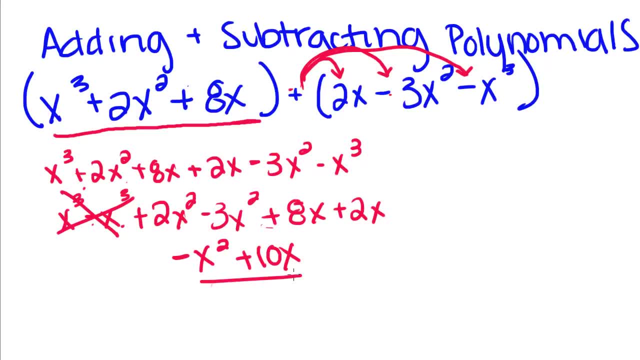 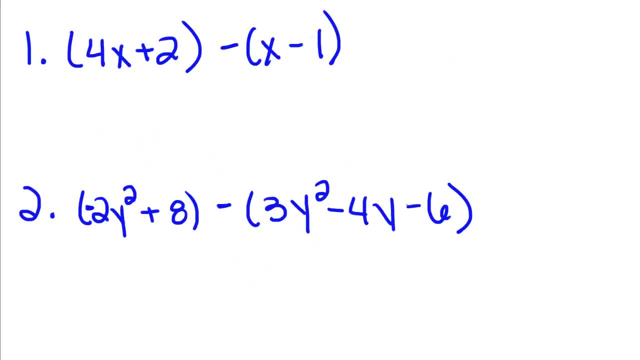 all you have to do It's really just Distribution and combining like terms. So we're going to do some examples now. Okay, so this time we have a negative. So it's really, really important that we distribute that negative because, if you forget, you're going to end up maybe adding some things that you're not. 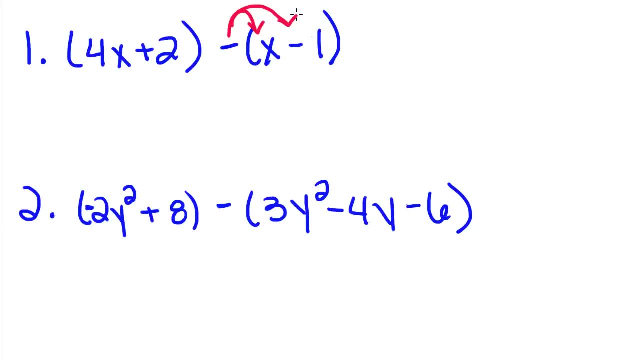 supposed to, or subtracting some things that you're not supposed to. So we're going to copy the first part. that stays the same. And when we take negative 1, because we're going to use a positive 1, it's the same. but we're going to re-cuadrate trues, breathe it. 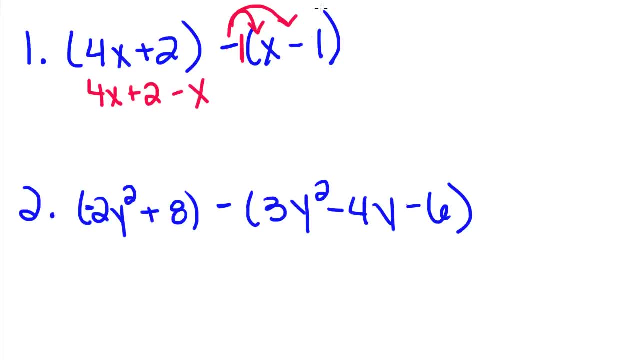 down. So now you're going to have negative x squared plus negative x squared plus 0.. 0 goes to 4x squared minus 1, and we have negative x squared minus 3x squared plus two plus one. that's a convertible, So we're going to add that up. We do our. 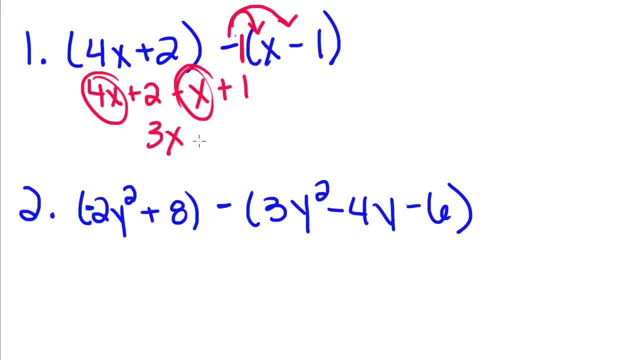 things by dividing. so we say: 3x squared plus negative 1 times x, squared plus 1 times negative, 1 is going to give us a positive one. So then we're going to combine our like terms: 4x plus a negative, x is going to give us 3x, and 2 plus 1 is going to give us 3.. Now if 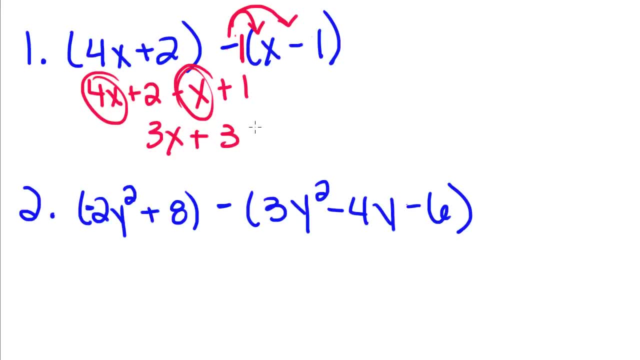 you remember, when I introduced these, I said they are in expression, So that I said that, And an expression is just what we call something that doesn't have an equal sign, Because if this said equals 9, then that would be an equation. 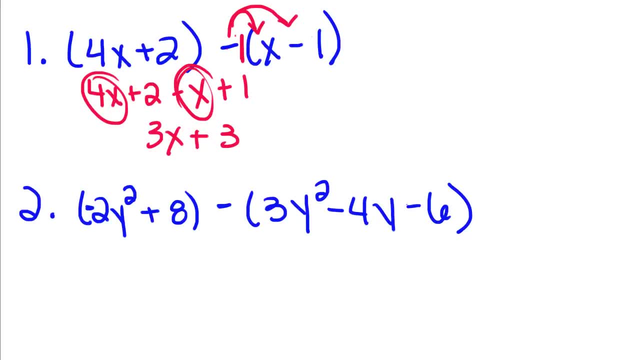 But when it doesn't have an equals, it's called an expression. Just in case you see that on homework or any other kind of worksheets that you do at home, I want you to know that that's all it means. So we're going to do the same thing down here: distribute this negative. 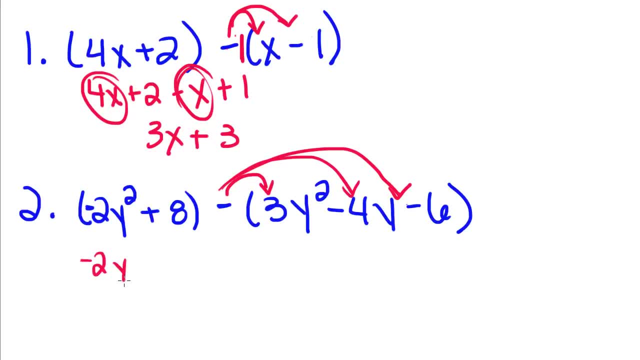 And that's really the most important part- is that if you have a negative, or even if, say, you had like a 2 right here, you'd have to multiply it all out so that you don't add or subtract incorrectly. So negative 2y squared plus 8, and that 2's not supposed to be there. 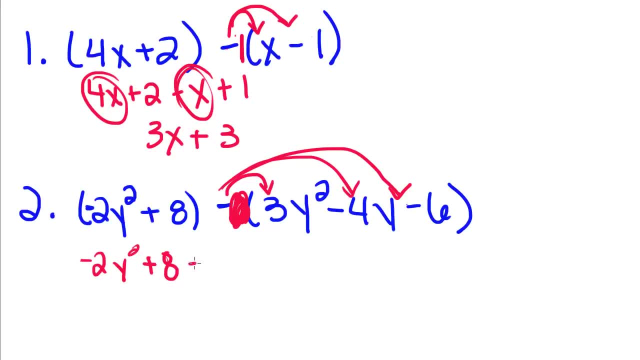 negative 1 times 3y squared is going to give us negative 3y squared. Negative times negative is going to give us positive 4y, And the negative times the negative is going to give us a positive 6.. Now we're going to combine our terms. 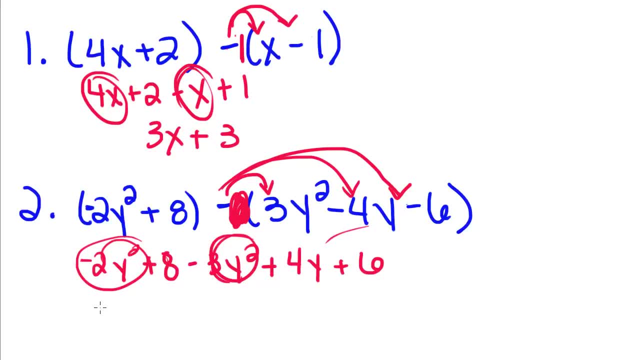 Negative 2y squared minus 3y squared is going to give us a negative 5y squared. And then we have a plus 4y because this- there's nothing else with a y in it, And then we have 8 plus 6.. 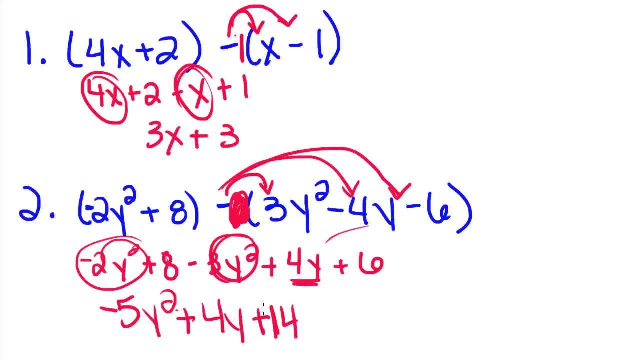 So plus 14.. So if you notice right here, this says 8 minus And there's a positive over here And you might not understand why I added 6 instead of subtracting 6.. But remember when we did some basic algebra. 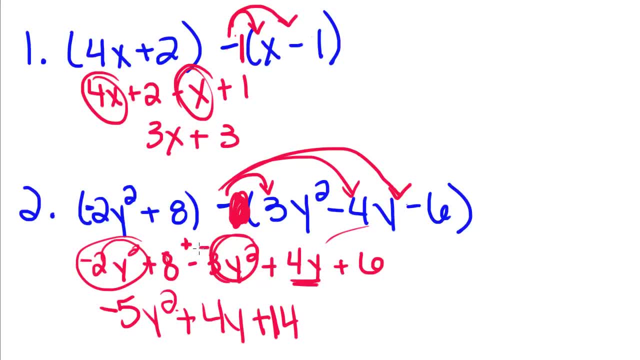 and we said that this is the same thing as adding a negative. well, that negative stays on that 3. It doesn't go with the 6. So you, that's you- really have to make sure that you pay attention to your signs.